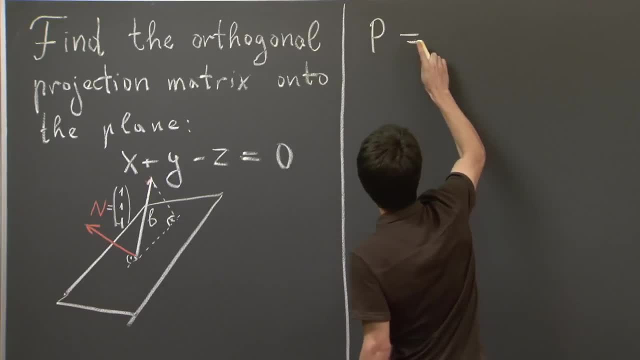 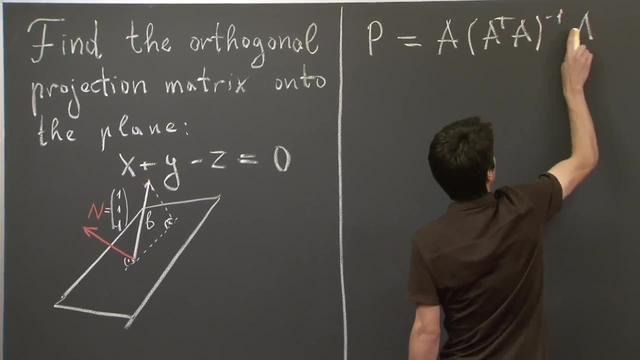 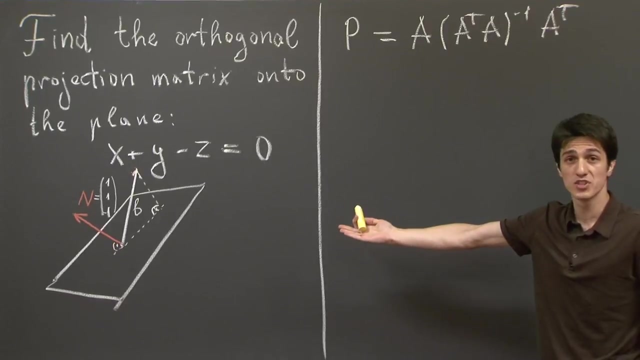 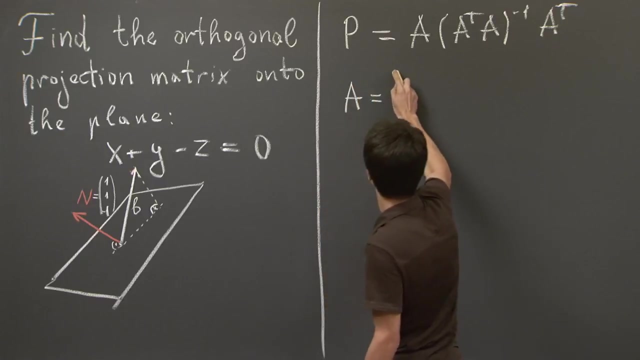 Well, slightly complicated expression. It's A times A transpose, A inverse A transpose, where A is a matrix that somehow encodes the subspace we are projecting on. Yeah, in particular, A has its columns A1, A2, I'm going to denote them: a basis, 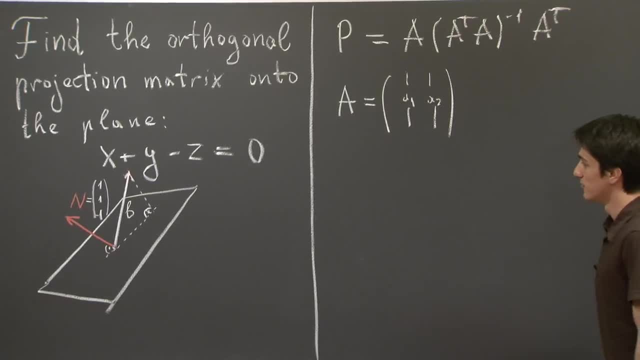 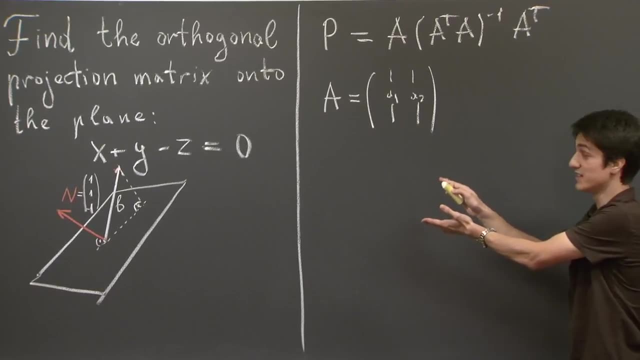 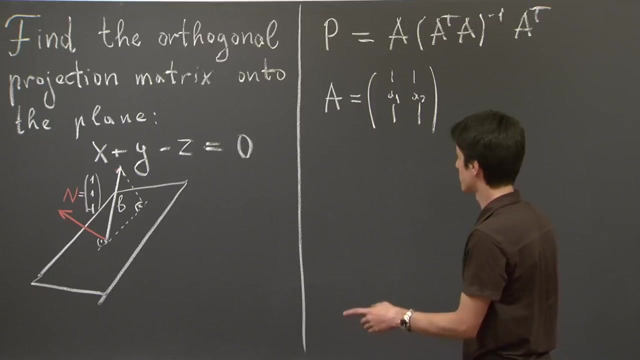 for the plane we're projecting on. So essentially, what we need to do is find two such vectors that span the plane and start computing with the matrix. Yeah, this is fairly straightforward. One choice that works, for example, is 1, negative, 1, 0 for the first column. 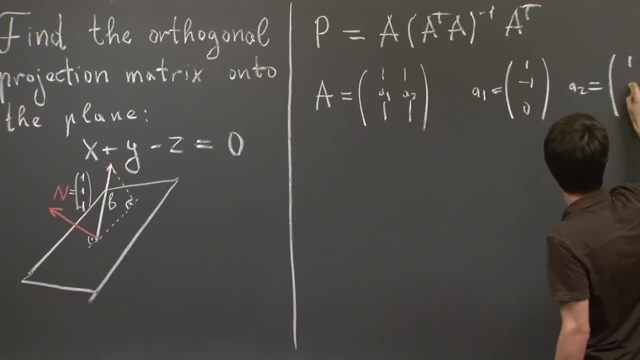 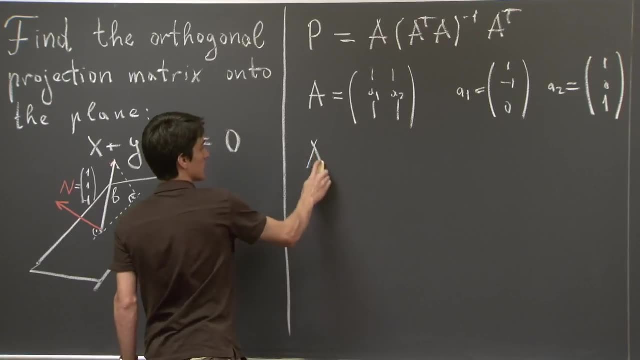 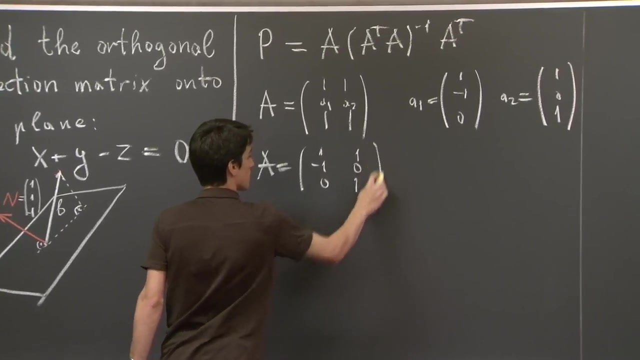 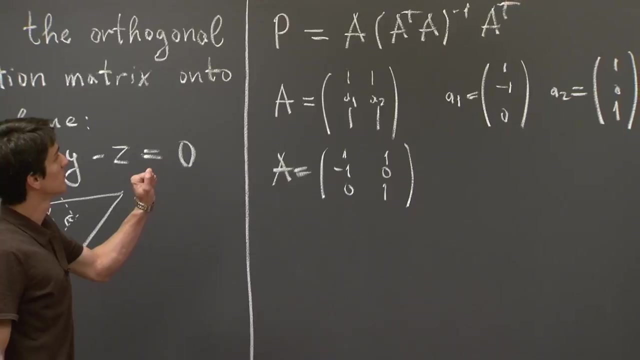 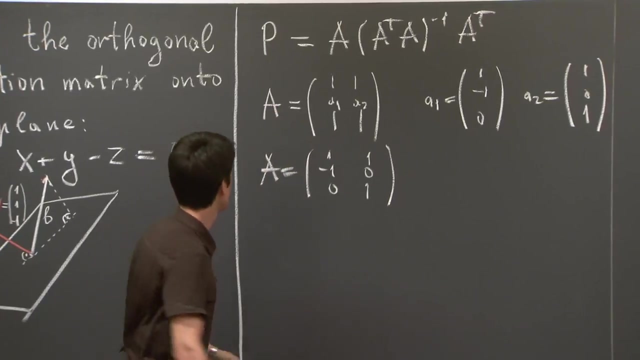 and 1, 0, 1 for the second column. OK, And let me write out the matrix A. OK, So in the formula I guess the slightly more complicated combination is A transpose, A inverse. So let me compute that first for you. 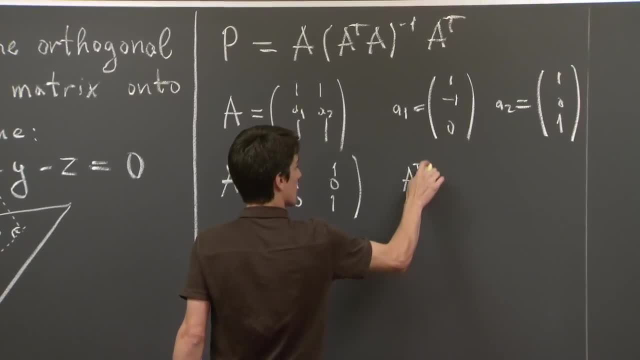 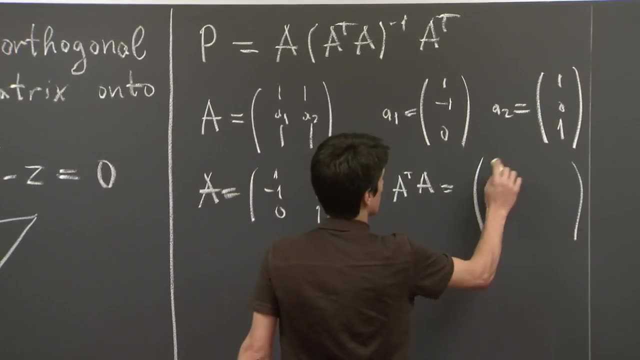 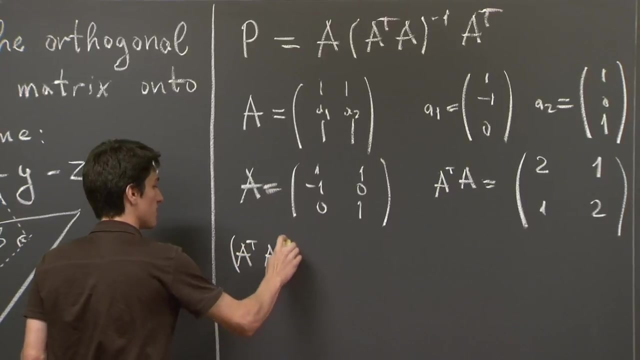 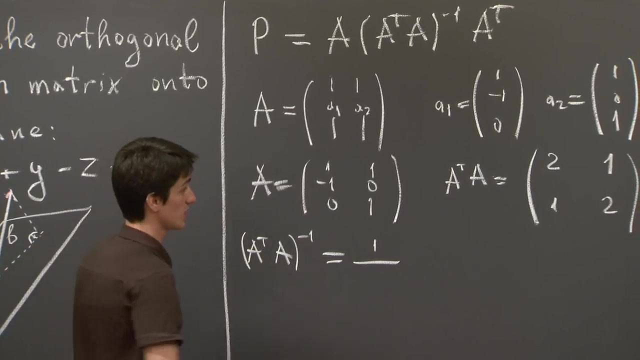 OK, So A transpose A is a 2 by 2 matrix, And it's not so hard to figure out. it's like 2 and 1, 1, 2.. OK, Now we shall invert it Using the familiar formula 1 over the determinant. 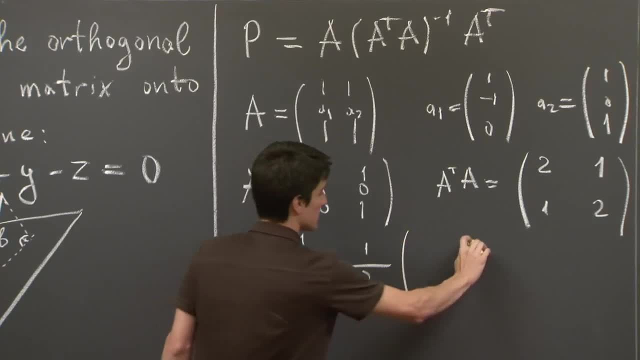 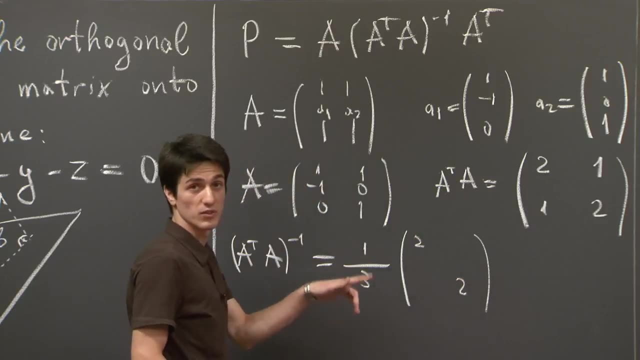 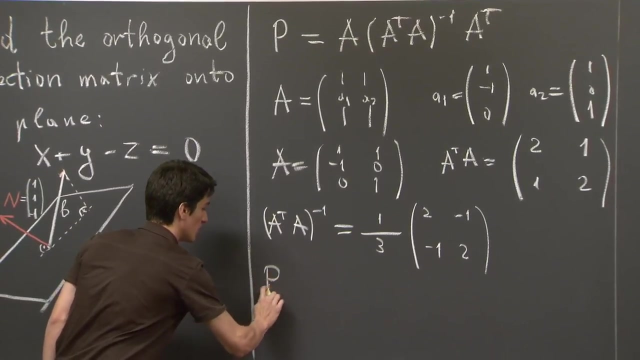 2 times 2 minus 1 is 3.. And so we switch the diagonal entries And we flip the signs of the odd diagonal ones. OK, Right, And therefore the projection matrix is given by default. OK, OK, OK. 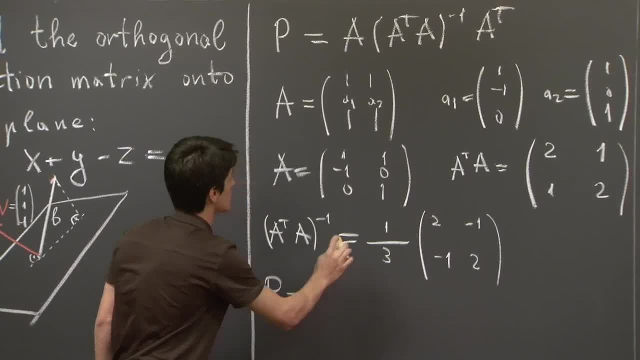 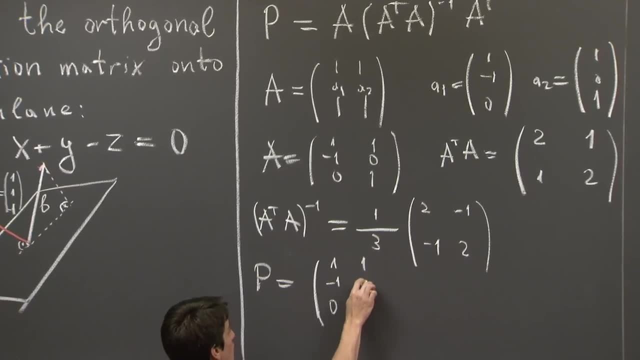 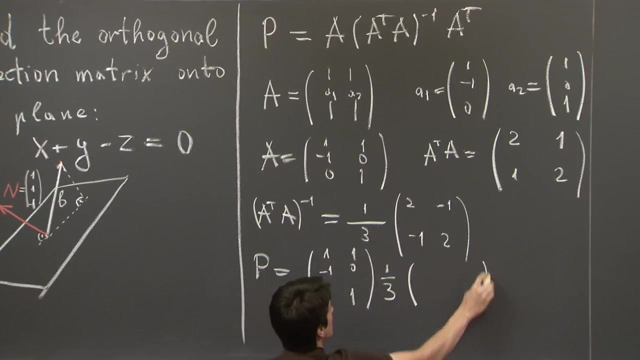 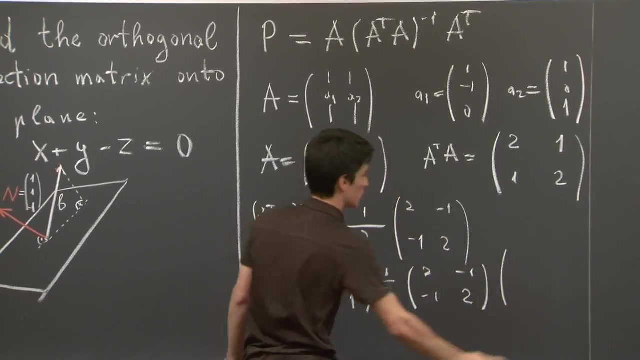 So we have the following product of matrices: 1, 3, 2, negative, 1, negative, 1, 2.. And then transpose of A, which is 1, negative, 1, 0, 2.. OK, 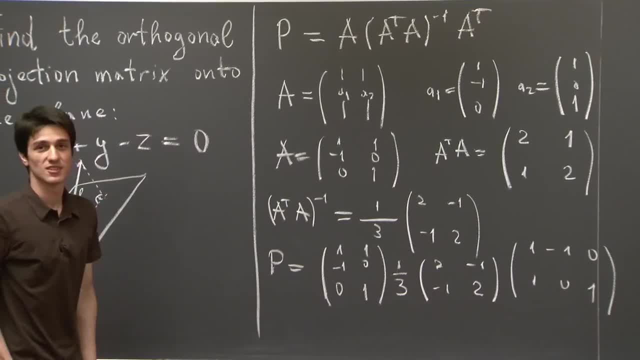 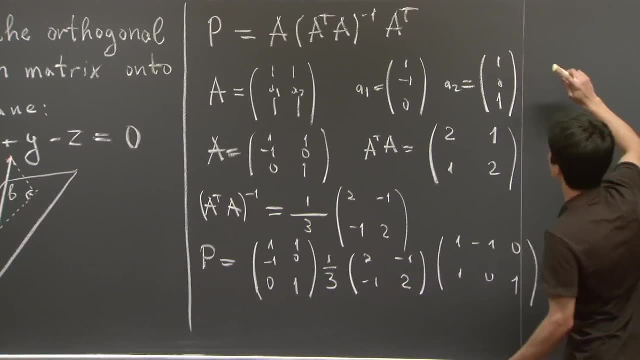 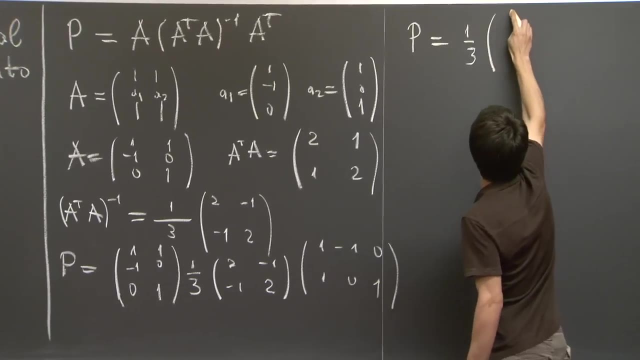 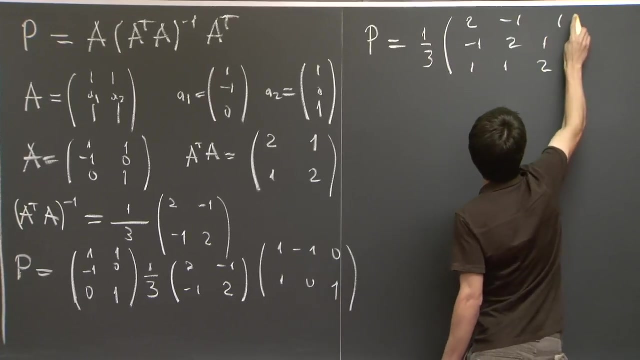 OK, OK, 1, 0, 1.. OK, I'm going to carry out this multiplication in an inhumanly fast fashion, So I'm just going to write down the answer, which is: 1 third, 2, negative, 1, 2, 2, 1, 1, 1.. 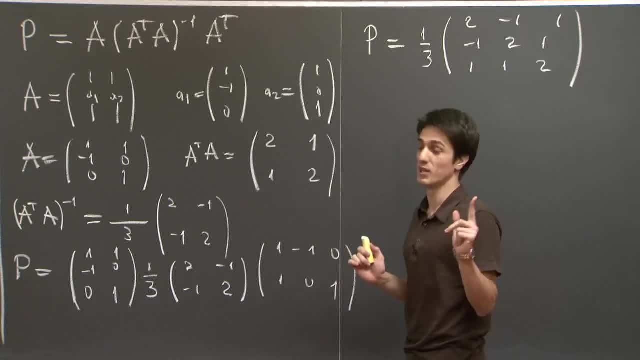 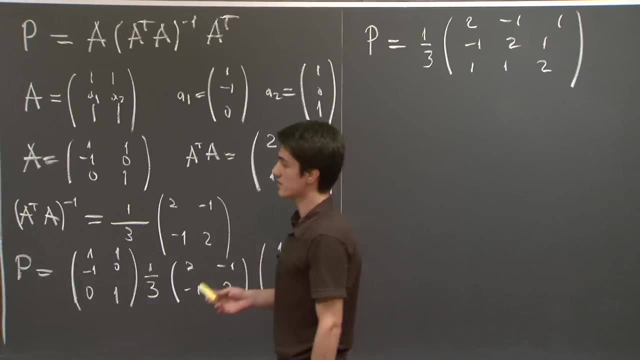 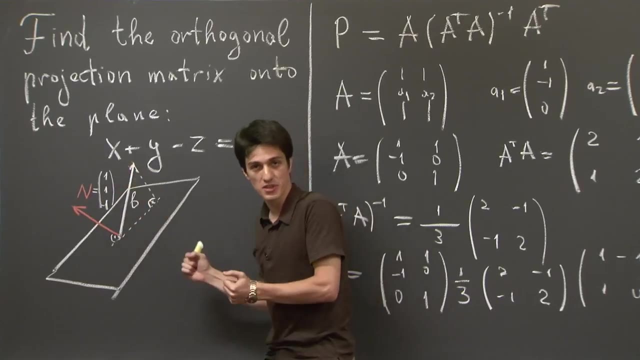 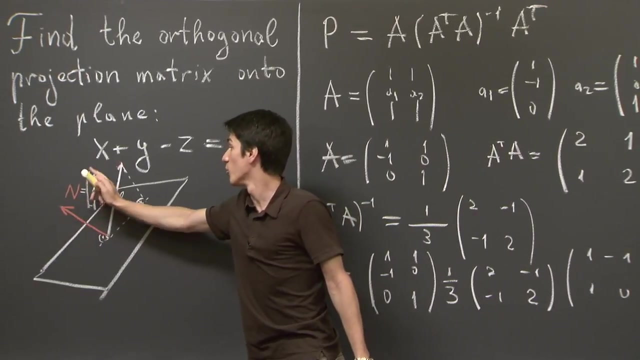 Right. So what you can do now is: well, you can check whether this answer actually makes sense. One thing you can do is just well, a projection matrix is supposed to take the normal to the plane down to 0. So you can just multiply p and the normal vector 1, 1,. 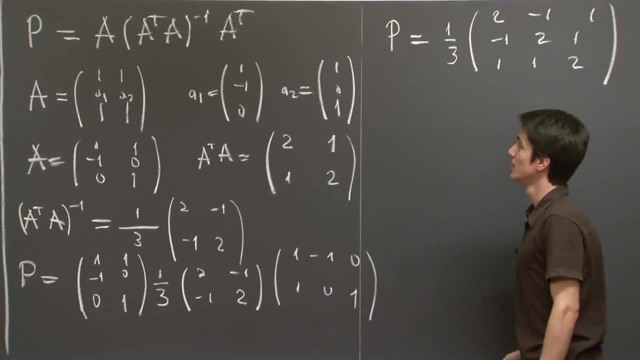 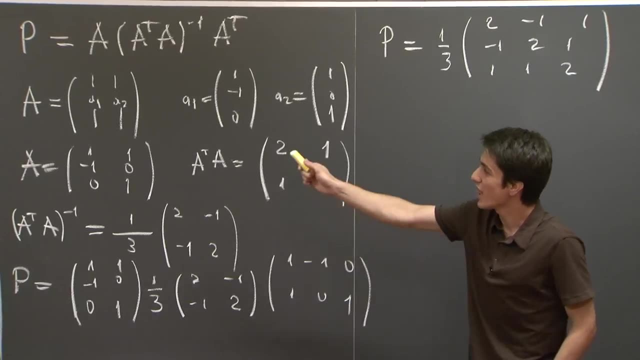 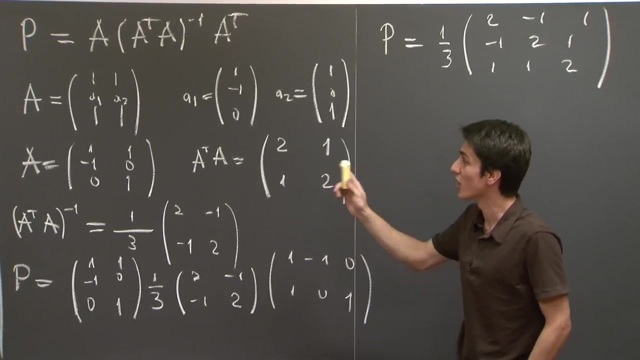 negative 1, and if you get 0,, maybe you've done a good job. Another curious thing that I would like to point out here is: so you see, we had lots of freedom of choosing the matrix A. I mean we could have chosen any two columns that. 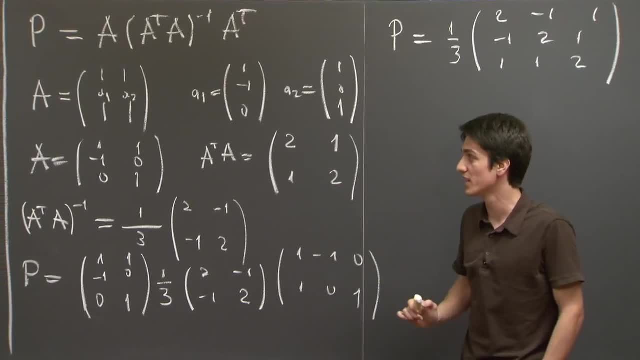 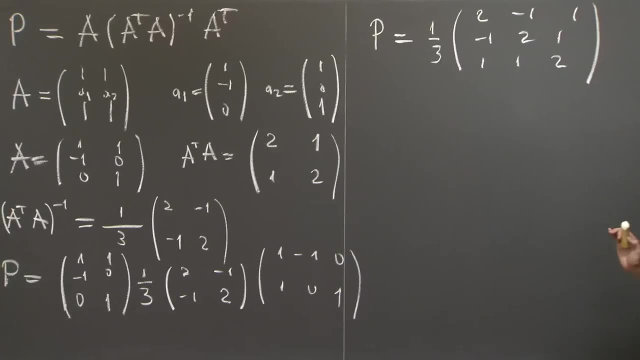 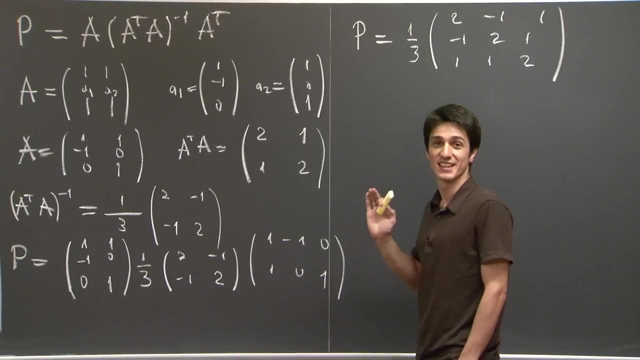 span the subspace that spans the plane. The beautiful thing about it is that in the end we would get the same answer Right. So I hope there will be many of you who would say: OK, Hey, There is an easier way to the problem. 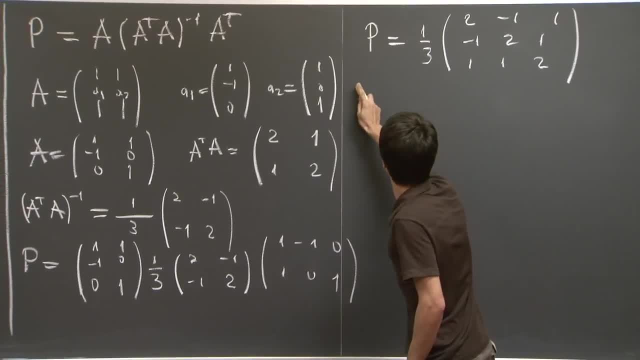 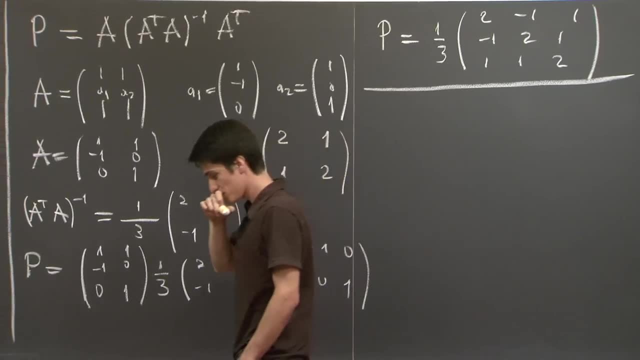 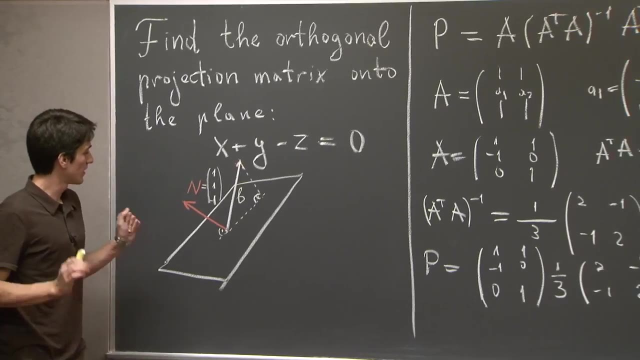 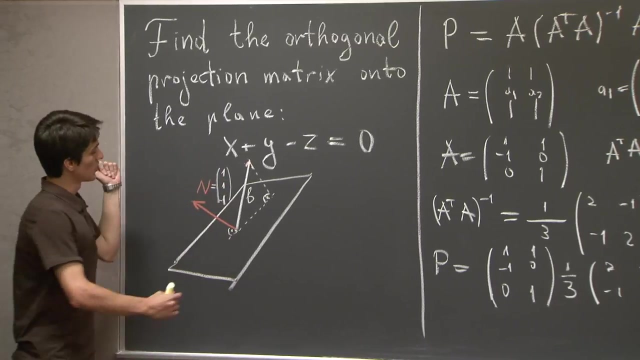 And I'll agree with these people. So let's see what would be an easier approach. Well, let's go back to the sketch here And let's make the following observation: that any vector is a sum of two components. The first component is: 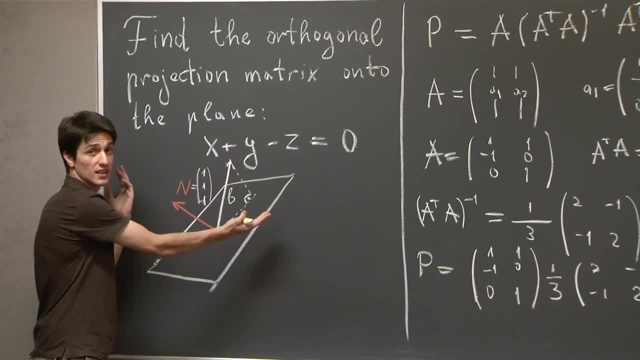 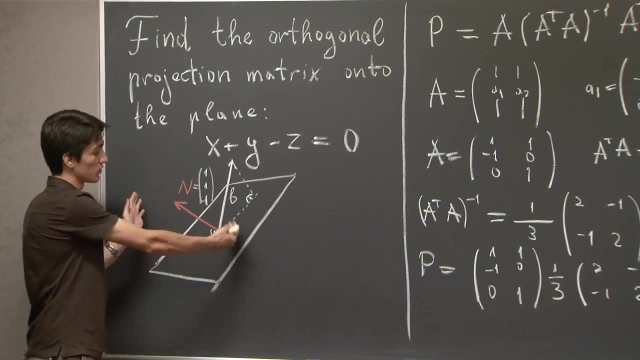 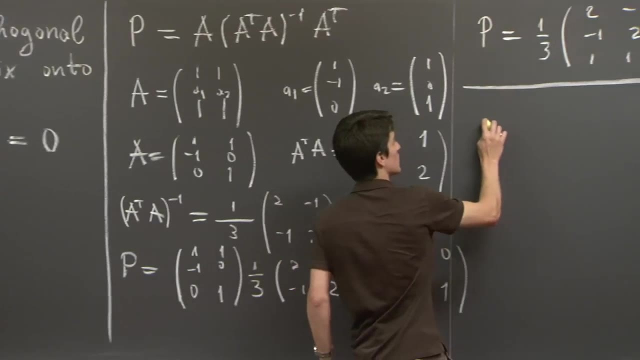 It's projection onto the plane, And the other component is its projection onto the orthogonal complement of the plane, In this case onto the normal vector to the plane. So in the language of linear algebra this is just b equals to its projection onto the plane. 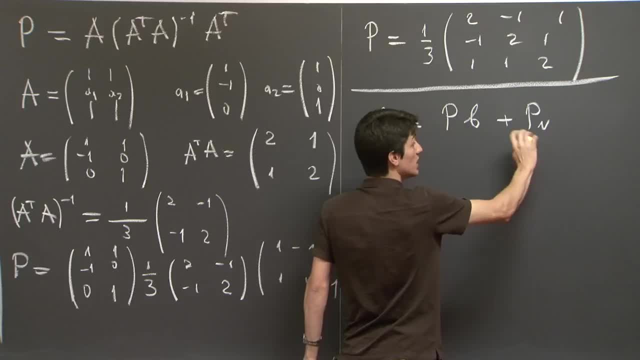 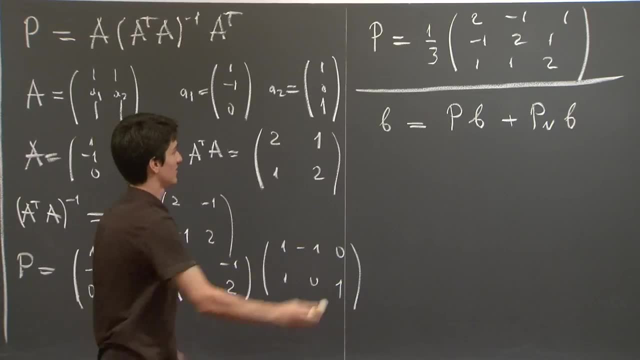 plus its projection. we're going to call it pn onto the orthogonal complement, So it's just b equals to its projection onto the plane. OK, I'm going to suggestively write here the identity matrix so that you can immediately read off. 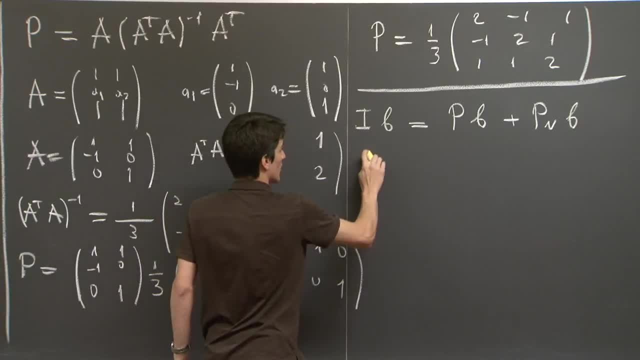 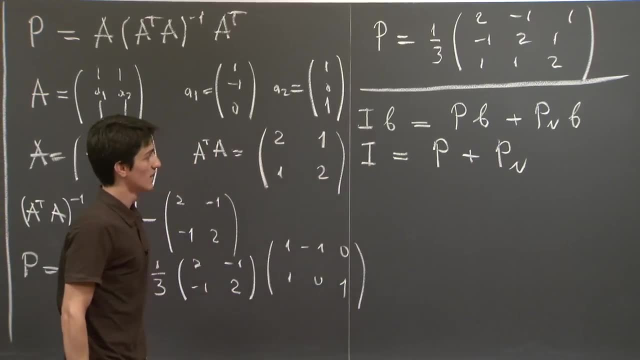 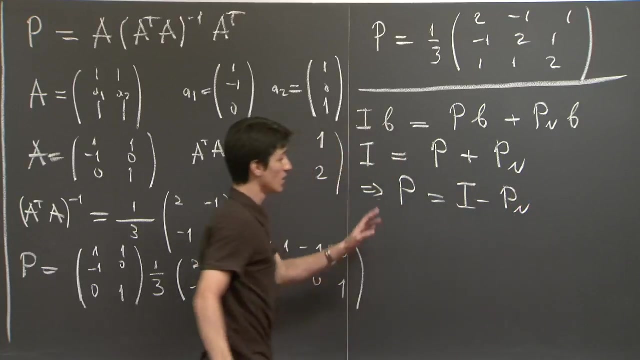 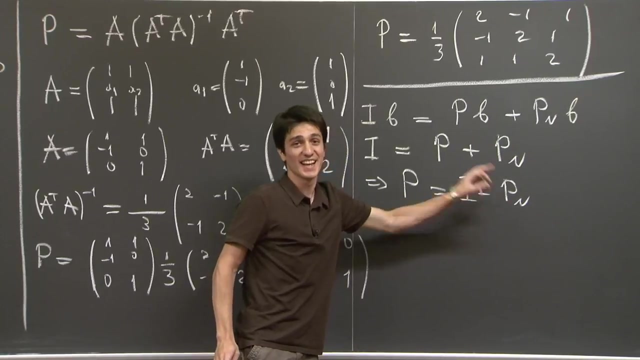 a matrix equality associated with this Equality. here it's: the identity equals p plus pn And therefore the projection matrix is just the identity minus the projection matrix onto the norm. This is the normal vector. Now this object, here pn, is much easier to compute. 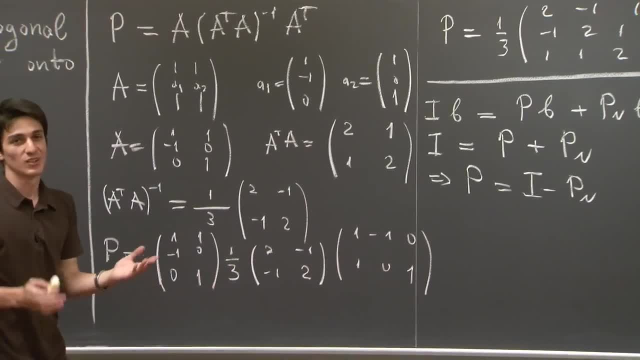 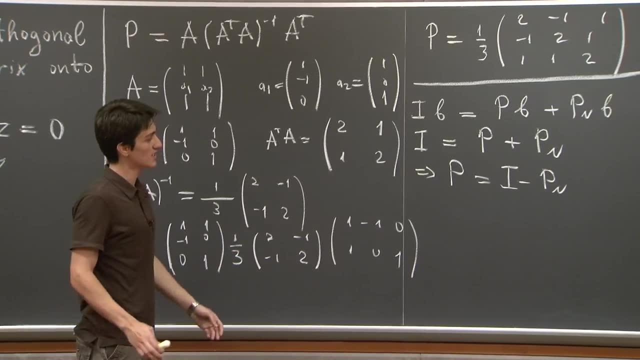 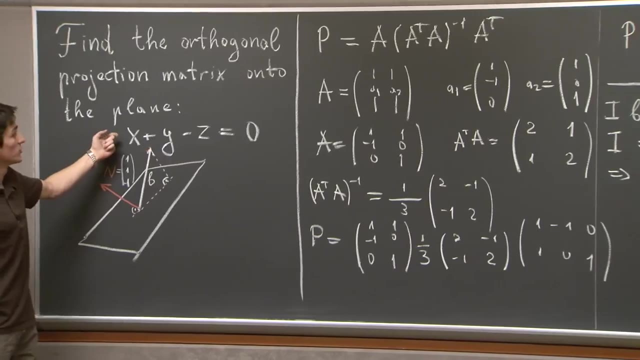 Well, for two reasons. First, one is that, well, projecting onto a one-dimensional subspace is infinitely easier than projecting onto a higher dimensional subspace. And second, we already have immediately, we can read off from the equation of the plane. 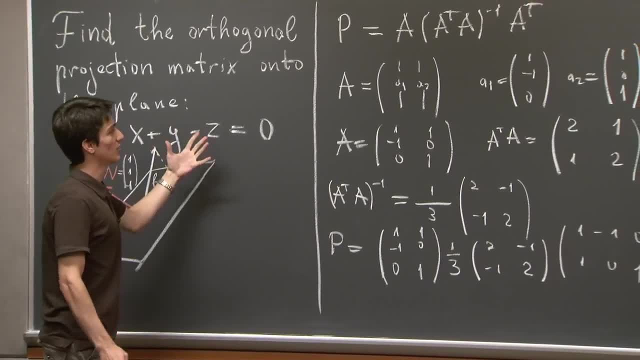 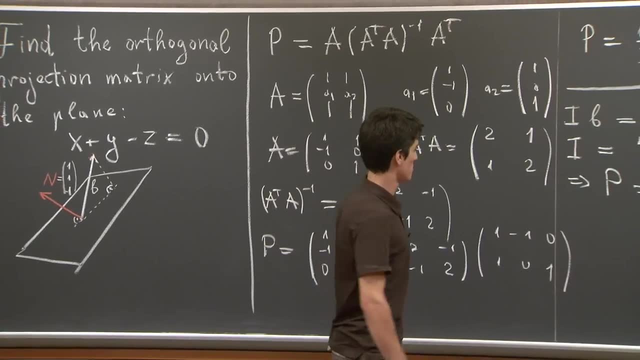 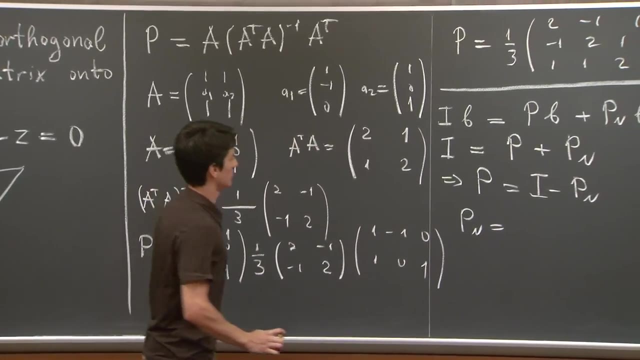 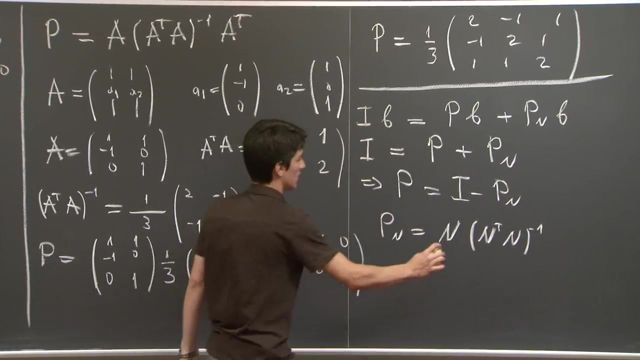 what the normal vector is. So we don't have to worry about that. OK, We don't have to derive these guys, Like we don't have to do what we did here. OK, So essentially pn will be n, n transpose, n, inverse. 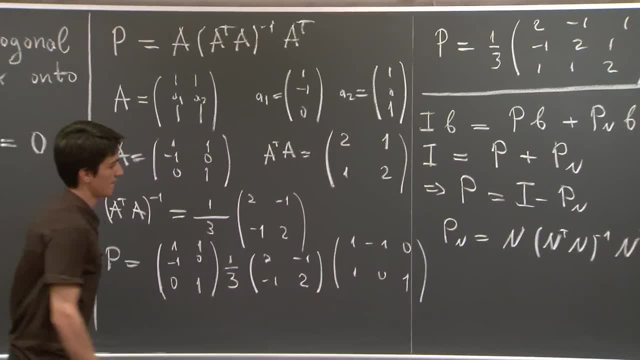 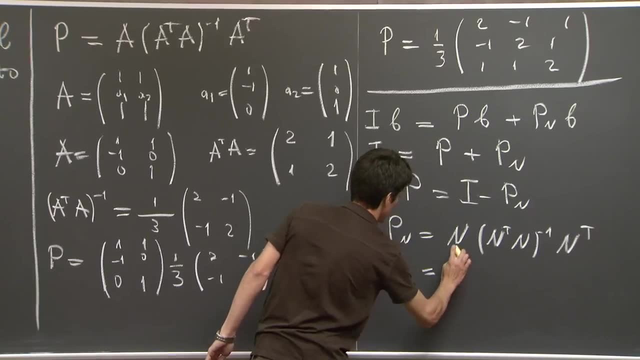 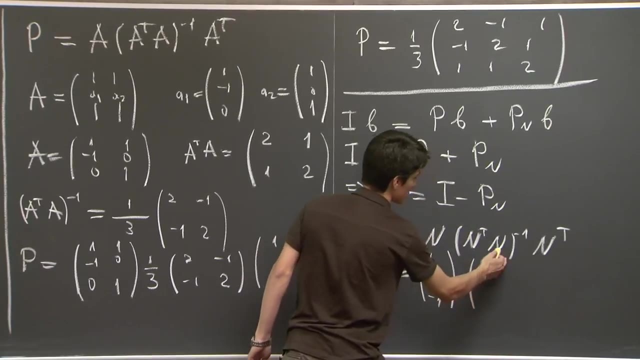 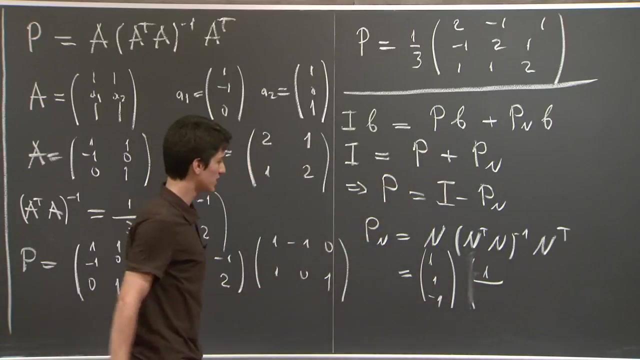 n transpose, And that's equal to 1, 1, negative, 1.. And n transpose n inverse. this is just a number. It's 1 over the magnitude of the normal vector. So that's the magnitude squared, That's 3..